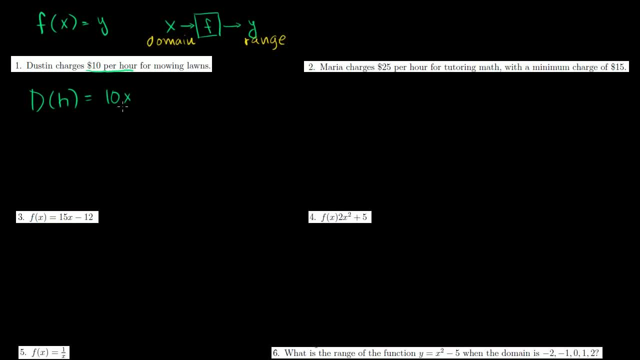 It's going to be 10.. Times: I won't write the times there. We know I could just write 10h And of course he can't work negative hours, So we could write. h is going to be greater than or equal to 0.. 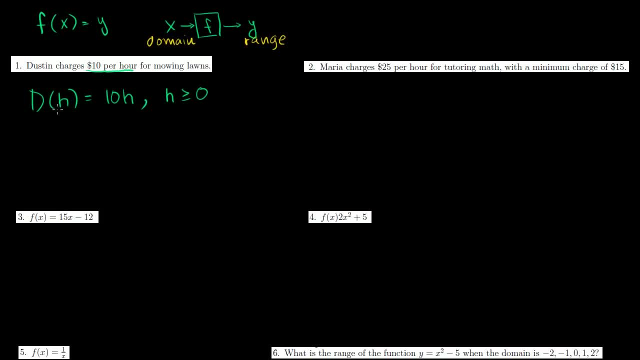 That's our function definition. If you say, hey, how much is he going to charge for working half an hour, You put 1 half in here, which essentially substitutes this h with the 1 half. You do 10 times 1 half. 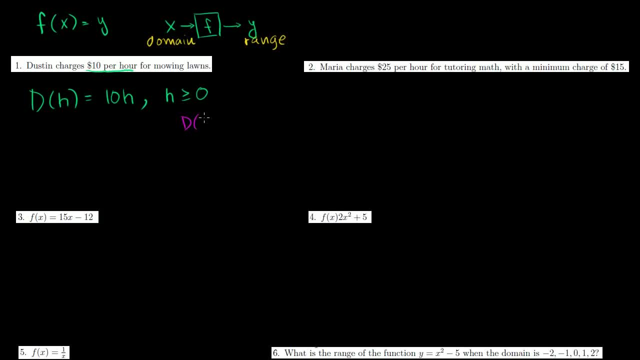 Let me write that down on the side here. So Dustin's going to charge for 1 half, He's going to charge 10,. wherever you see the h, replace it with 1 half times 1 half, which is equal to $5. 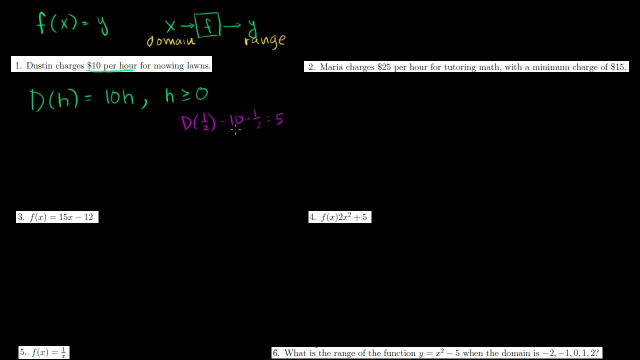 That's our function definition. I was just showing you an example of applying it. Now let's figure out the domain and the range. So I almost explicitly say it here: You can't work negative hours. This number, this function is not defined if h is less than. 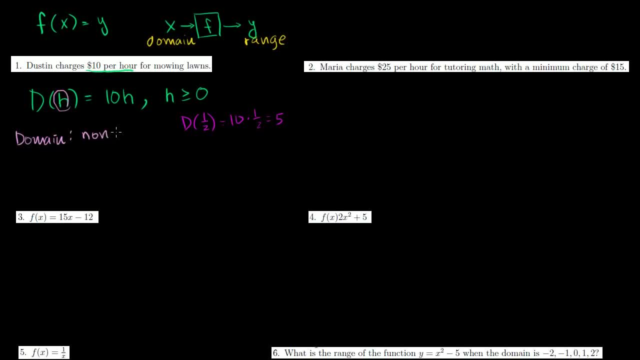 0.. So we could say non-negative and we could say real numbers, which could be everything, including pi and e and all of that. but you can't legitimately charge someone 10 times pi dollars. That's not a legitimate amount that one can charge someone in. 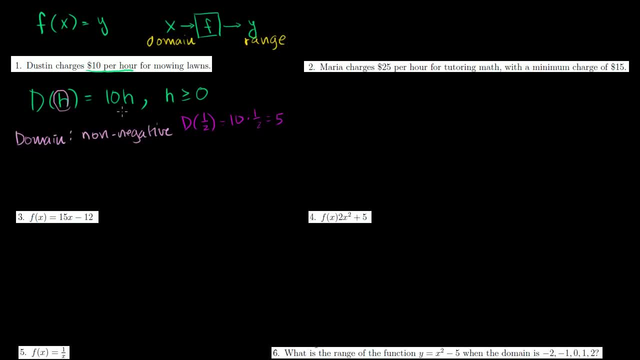 the real world because at the end of the day you have to round to the penny. You can't actually charge them that. So any number that he charges is going to be a rational number. It can be expressed as a fraction, So we can kind of take out numbers like e and pi. 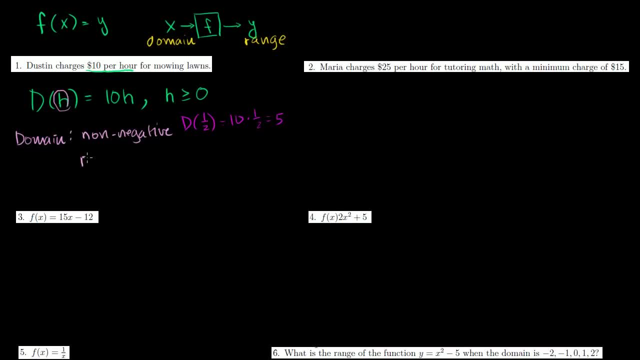 So, if we want to be really cute about it, we would say: non-negative rational numbers, And these are just numbers that can be expressed as a fraction, which are most numbers? just not these numbers that just keep not repeating, and all of that. 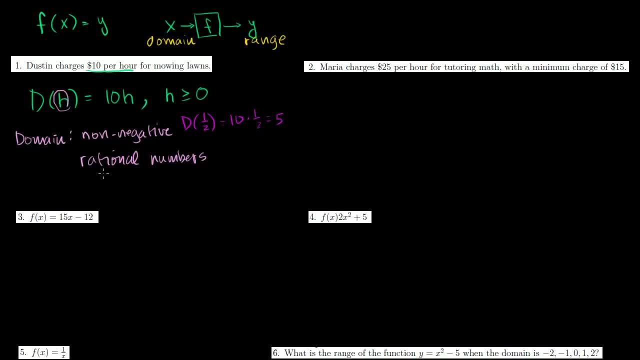 So non-negative rational numbers is what he can input in here, And then the range which is the valid the range. once again, whatever number you put in for h, remember you can only put in non-negative values for h- non-negative. 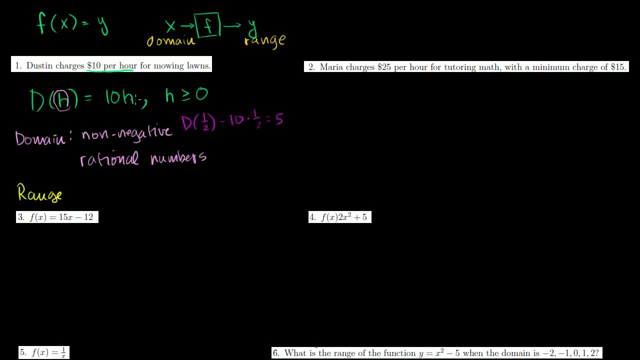 rational values for h. So whatever numbers you put in for h, you're going to get positive values for how much he charges for 10h, for the value of the function. So once again it's going to be non-negative. and if you put 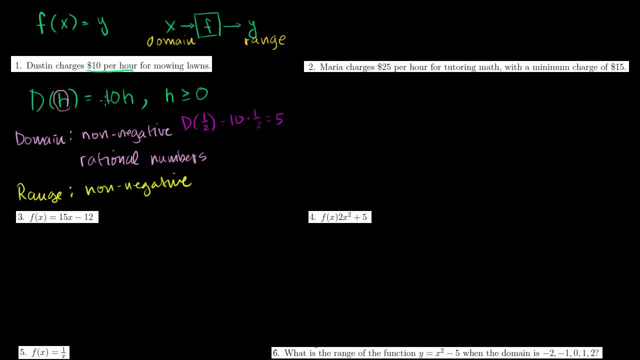 a rational number. here it's being expressed as a fraction. you multiply it by 10, it's still going to be a rational number, non-negative rational, And if you want to be really cute, you could say any number that can be expressed as dollar signs. 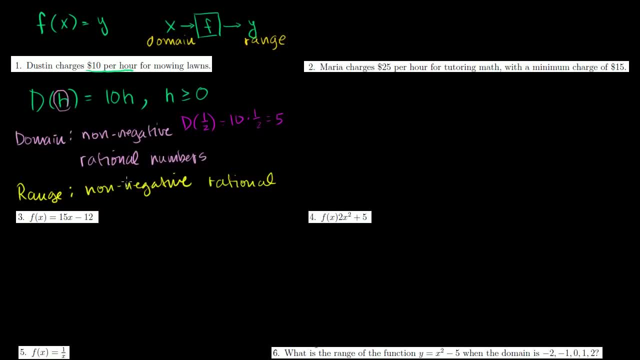 But anyway, I don't want to get too cute on this problem. I think you get the idea. Let's do more problems. All right, here we have Maria doing some tutoring. Maria charges $25 per hour for tutoring math with a minimum. 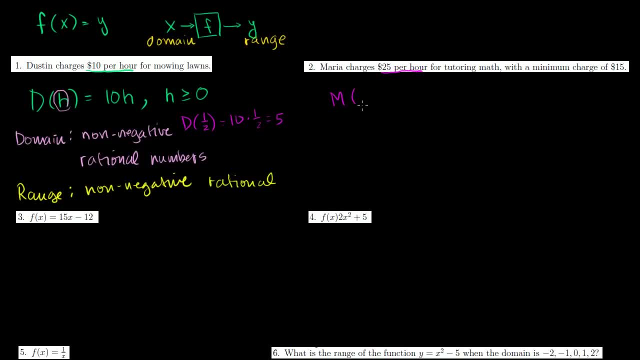 charge of $15.. So Maria charges as a function of hours, so she's going to charge $15 if you don't get enough hours in. So, at $25 per hour, in order to make $15, you've got to work 15 twenty-fifths, so that's 3 fifths of an hour. 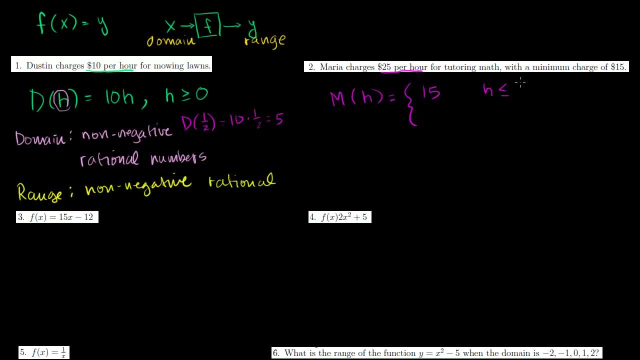 So if her hours are less than 3 fifths and greater than or equal to 0, she's going to charge $15. Because if she only worked 1 fifth of an hour, the bill would have been $5,. but she says she has a. 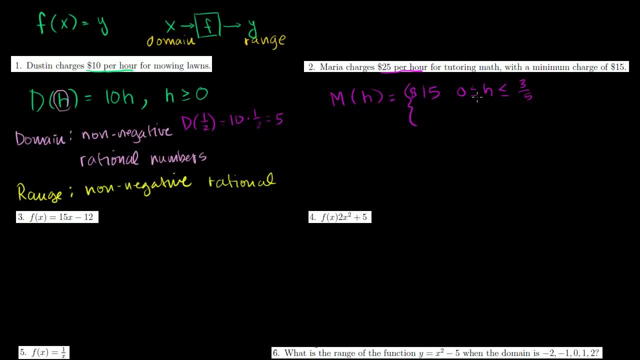 minimum charge of 15.. So she's going to charge $15 up until 3 fifths of an hour, or 36 minutes, And then after that, for h greater than 3 fifths, she's going to charge $25 an hour. 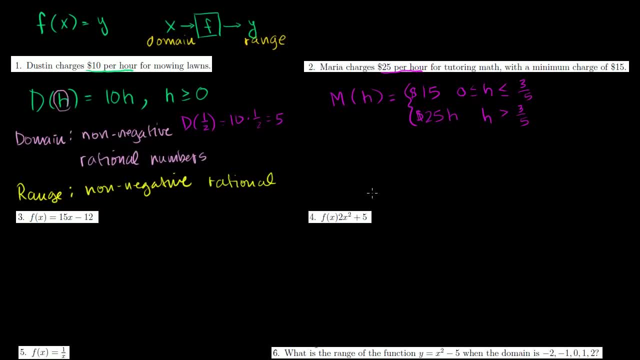 She's going to charge 25 times h. So that's her function definition, right there. Now, what is the domain? The domain for Maria's billing function? Well, let's see Once again. this is only defined for non-negative numbers, and by the same logic we used here, we got a little. 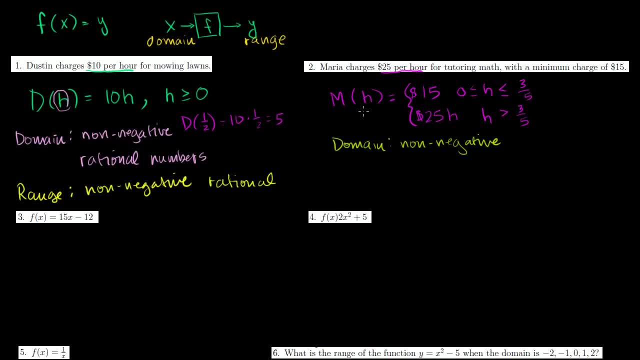 cute. we said: oh well, you really can't put, she really can't charge e hours or pi hours. That's not realistic for her to measure. Everything's going to be expressible as a fraction, For example, even 5,. if you say 5 hours, that's still a. 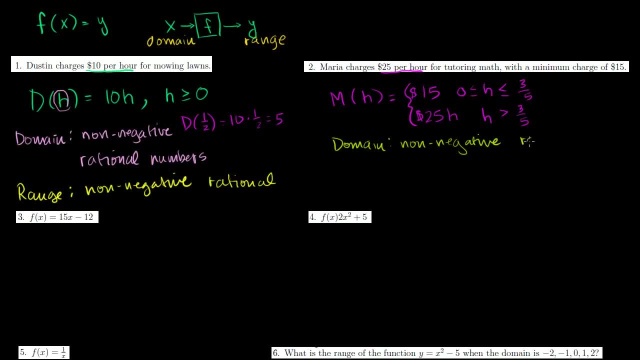 fraction, that's 5 over 1.. So we'll say 9.. That's non-negative rational numbers. And what's the range of her charging function or her billing function? Well, it has to be at least $15,, no matter what. 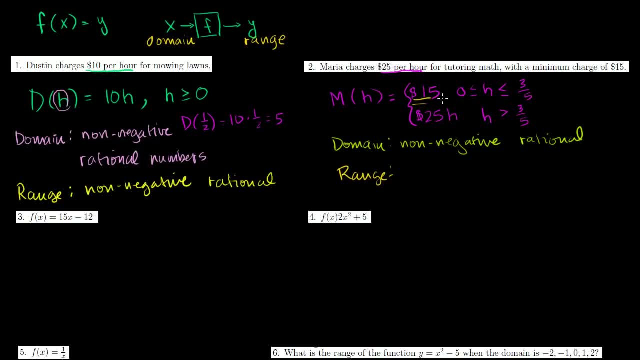 She's going to charge $15,, so it's going to be $15 or more, So it's going to be rational numbers greater than or equal to $15, right? There's no situation in which she will charge $14.. There's no situation in which she would charge negative $1. 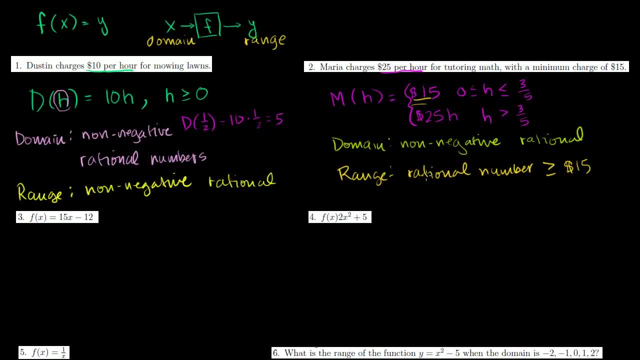 Everything's going to be greater than or equal to 15.. All right, so now we have these more abstract function definitions, so now we can stick really any number in it. Well, we're not going to deal with complexes, any real number, but let's see if they limit it a little bit. 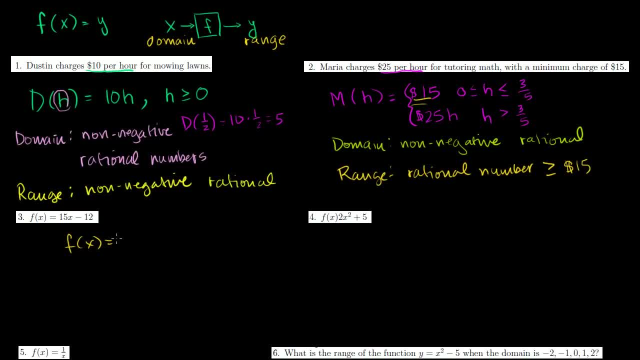 So we have f of x. let me rewrite it: f of x is equal to 15x minus 12.. So what's the domain? Well, I could stick any real number x in here and I'm just going to multiply it by 15 and then subtract 12.. 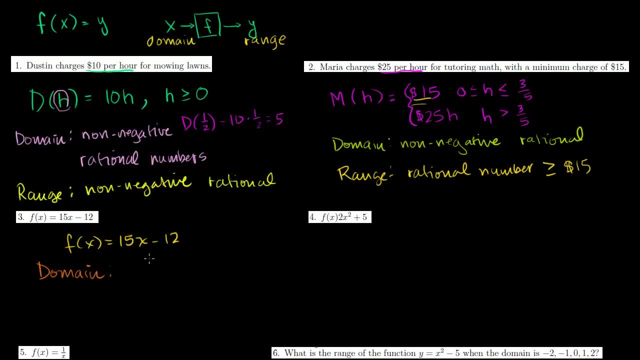 I could put pi there, I could put the square root of 2 there, I could put e there. I could do all sorts of crazy things. So I'm going to say all real numbers. Any real number I put in for x, I'm going to get a. 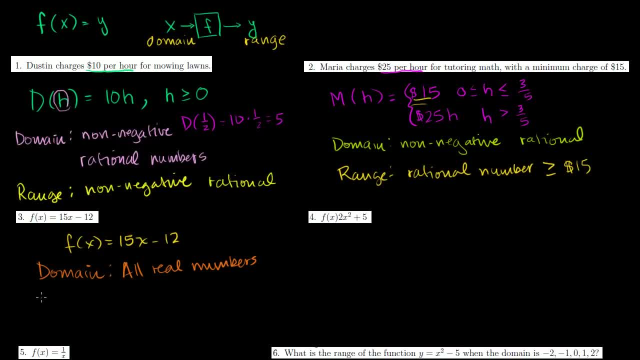 legitimate output. And then, what is my range? Well, once again, this can take on any value out there. I can get to any negative value. if I make x negative enough, I'm going to subtract 12 from it, but I can get to any. 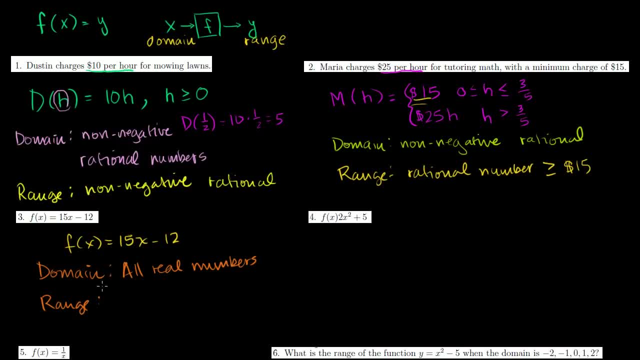 negative value. I can get to 0,. I can get to any positive value. so this is also going to be all real numbers. All right. now we have this function. It says f of x is equal to. they forgot the equal sign 2x. 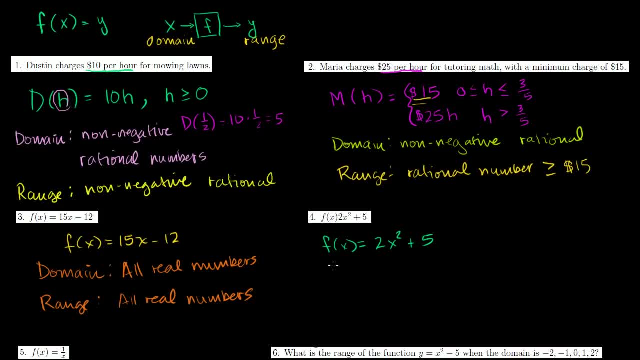 x squared plus 5.. So what is the domain? The domain, What are all of the valid values for x that I could stick here? Well, I could stick anything here. I could put e there 2 times e squared plus 5.. 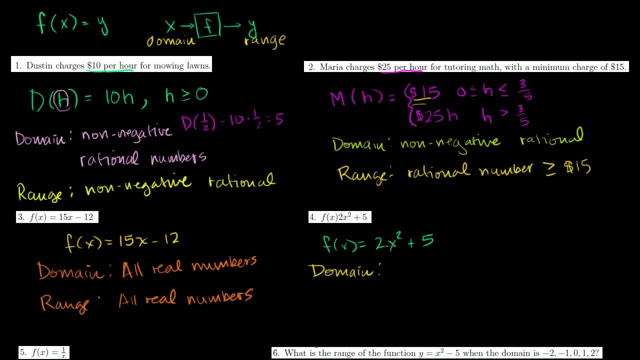 I could put a square root of 2 there, I could put a negative number there, So I could really take on any real number, all real numbers, positive or negative or otherwise, or even non-rational. And then what is the range here? 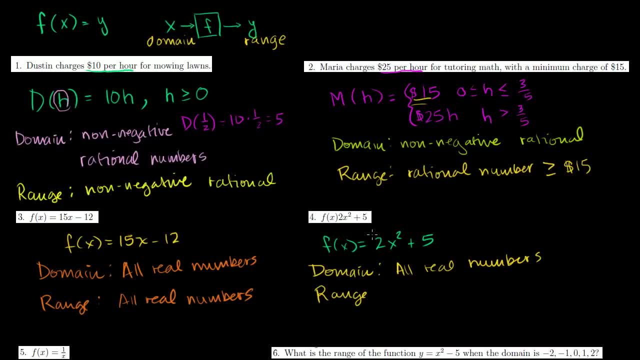 And this is interesting because no matter what number I put here, this value right here is going to be greater than 0. This is going to be right here, non-negative. Even if you put a really negative number here, you're going to square it. 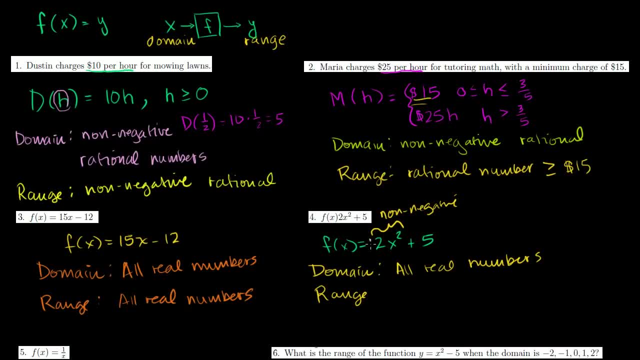 So it's going to become a really positive number when you square it. So this expression right here is going to be non-negative. So you take a non-negative. If you take a non-negative number and you add it to 5, you're always going to get something greater than 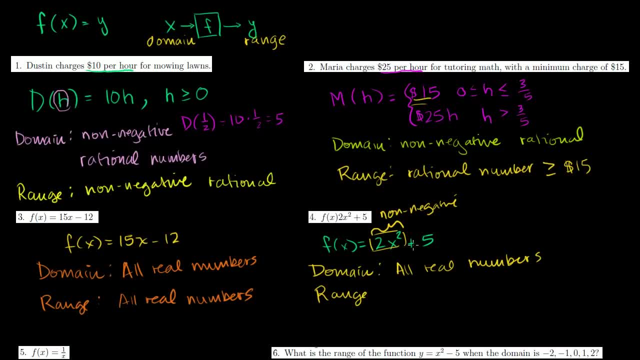 or equal to 5, right Worst case, this is a 0, and then you get a 5.. But if this is either slightly less than 0 or slightly more than 0,, you're going to get values greater than 5.. 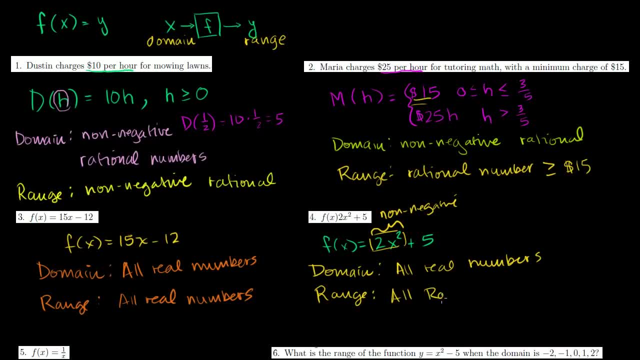 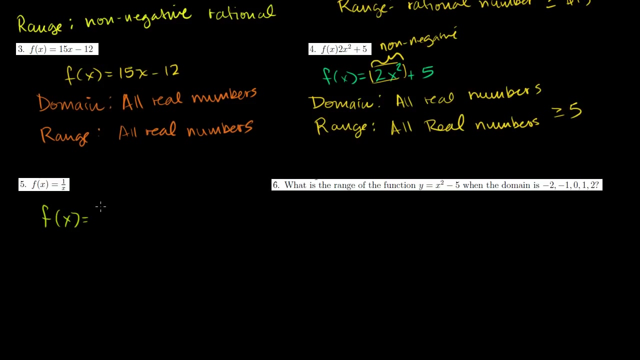 So the range is all real numbers greater than or equal to 5.. Your f of x could never take on the value 0. There's no way to get 0. Problem 5.. Problem 5. They have f of x is equal to 1 over x. 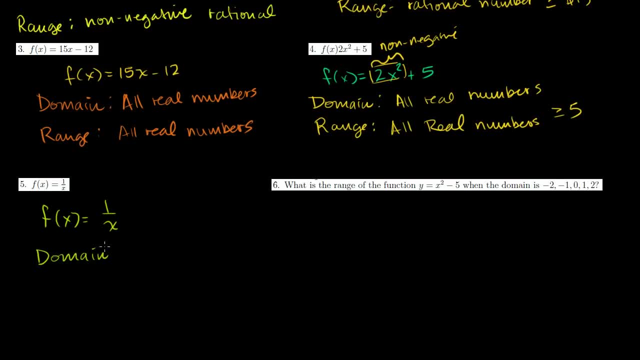 So once again, our domain. Well, we could put any value in for x. Any real number will work for you. We're just going to take the inverse of it. So this is going to be all real numbers. And then, what is the range? 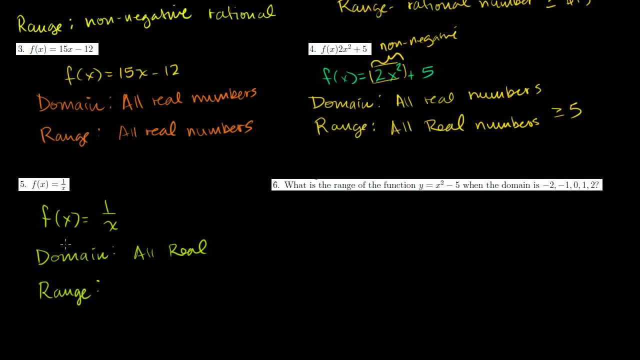 And this is interesting as well, Because, no matter what I put here, if I can put anything here, oh actually, let me be very, very careful. This is not defined, for x is equal to 0.. All real, except all real that are not equal to 0.. 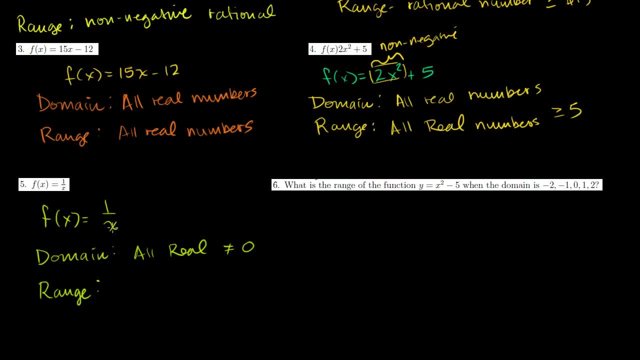 If I put 0 here, I'm going to get 1 over 0. It will be undefined. Let me write that down. I almost made a mistake. f of 0 is undefined And that literally means we don't know what to do with a 0. 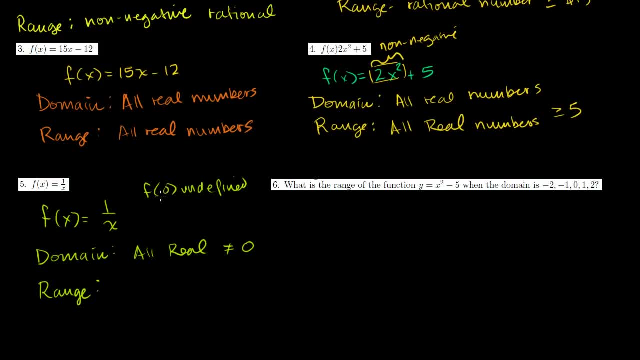 We have not defined a way to undefine. We operate on a 0. So f of 0 is undefined. So the domain is all reals except for 0. And now, what's the range? Well, once again we can take on any value here except 0. 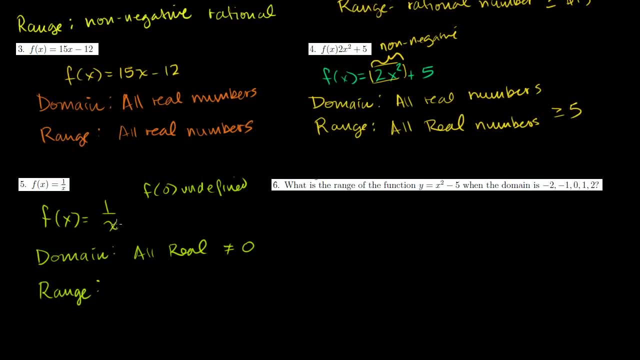 We could try to approach 0. If x got really really, really, really, really large, then this will become a approach 0. If x got really really negative, it'll approach 0. But in no circumstance will we actually ever get to 0.. 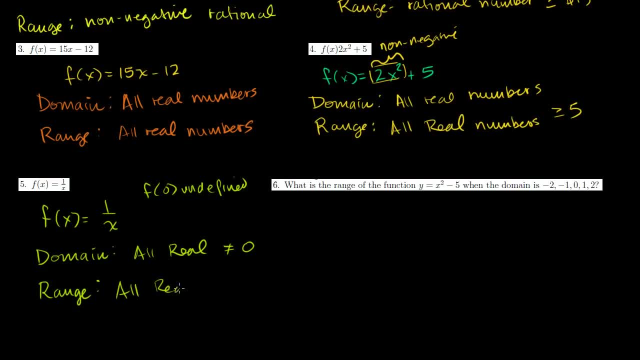 So, once again, all reals, All reals that are not equal to 0.. All real numbers except for 0.. All right, problem 6.. What is the range of the function? y is equal to x squared minus 5 when the domain is. 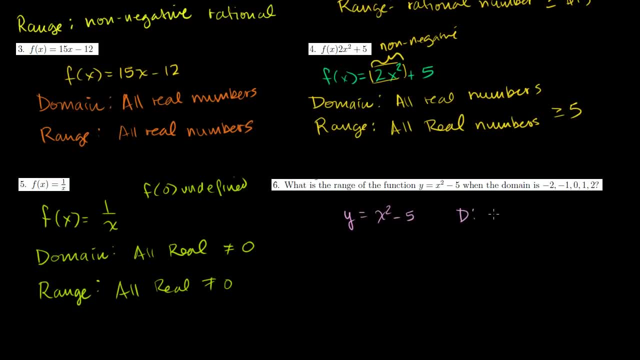 So they're defining the domain, They're restricting it, They're saying the domain is just the numbers minus 2, minus 1,, 0,, 1, and 2.. So this function definition really should say: f of 0 is. 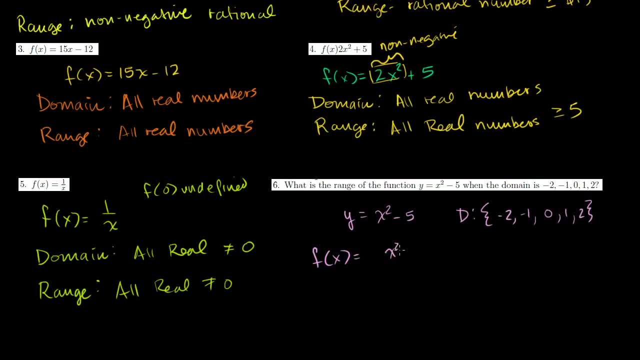 equal to x squared minus 5 for x is equal to: we could write: any member for x is a member of the set minus 2, minus 1, 0, 1, 2.. It's not defined for x being anything else than that. 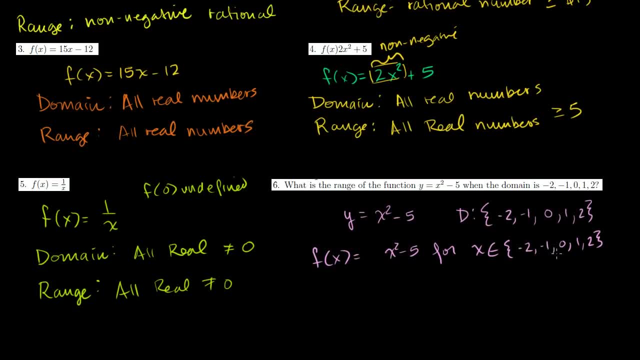 You don't know what to do with it. You can only apply it if x is one of these. So what's the range? Well, the range is all of the functions, all of the values that f of x can take on. So the range is going to be the set of values that we get when 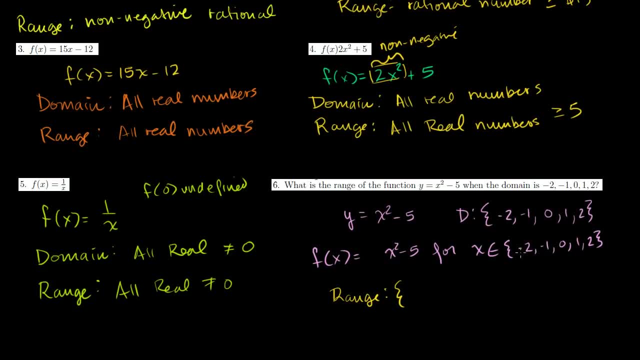 we put in all of these different x's. So let's try this first one: Negative 2.. Negative 2 squared minus 5.. Well, that's 4 minus 5.. That's negative 1.. Let's do negative 1.. 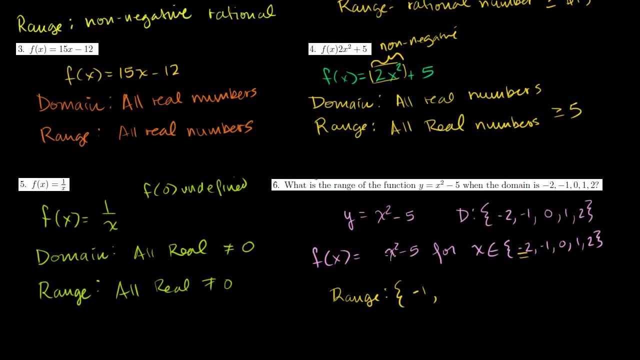 Negative 1 squared minus 5.. That is 1 minus 5.. That is negative 4.. You have 0.. 0 squared. So if f of 0,, you have 0 squared minus 5.. That's negative 5.. 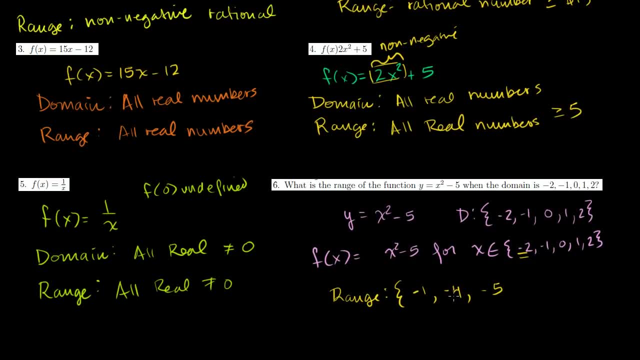 Then you have 1. 1 squared minus 5. Once again, that's negative 4. So it's already in our range. Then you have 2. 2 squared minus 5. That's negative 1. Already in our range.